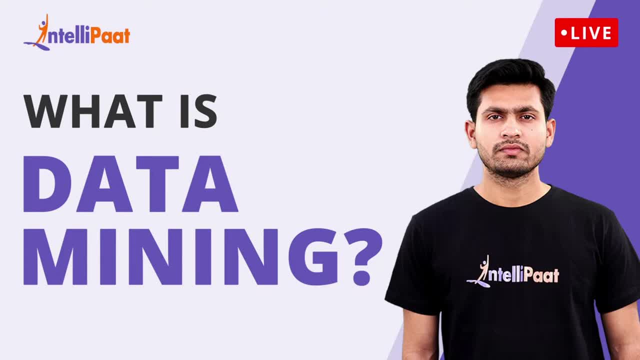 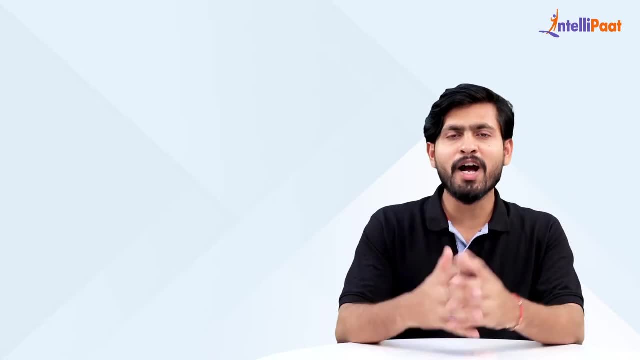 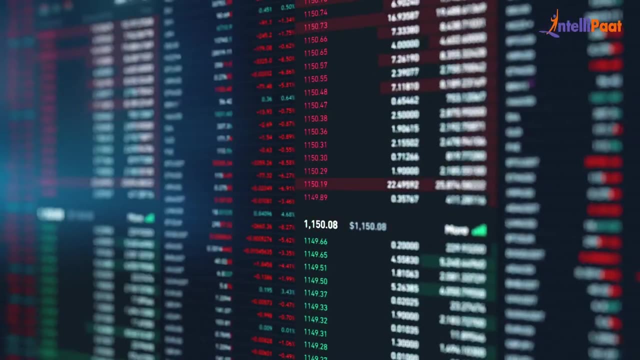 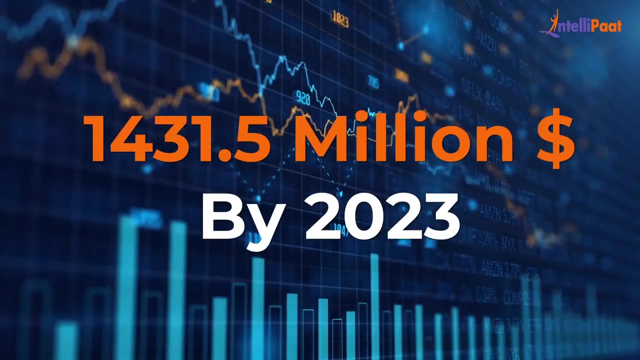 Hello everyone and welcome to today's session on what is data mining? Do you know, friends, that the global data mining market is expected to grow about 1431.5 million dollars in 2023?? After completing proper training and certifications in SQL data analysis. 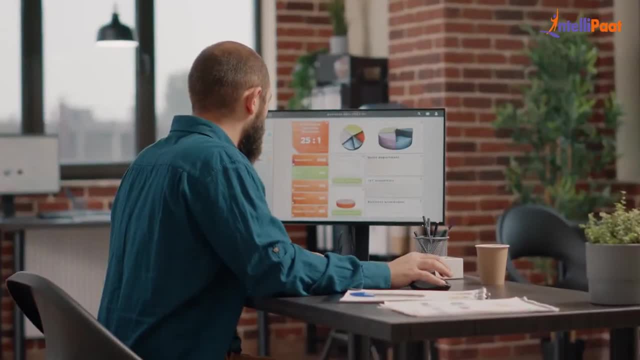 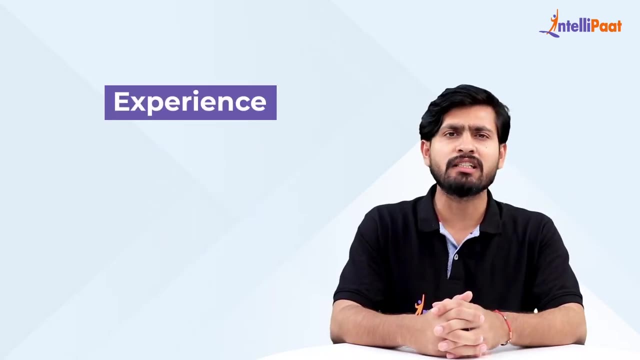 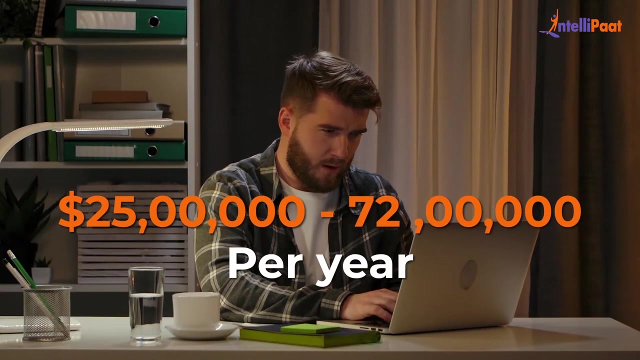 and statistical analysis. you can bag a job as a data mining analyst with average of 5.5 LPA per year, Depending upon your experience, your additional skills, location and employer. you can bag a job of around 25 lakhs per year to 72 lakhs per year- Very great numbers Sounds. 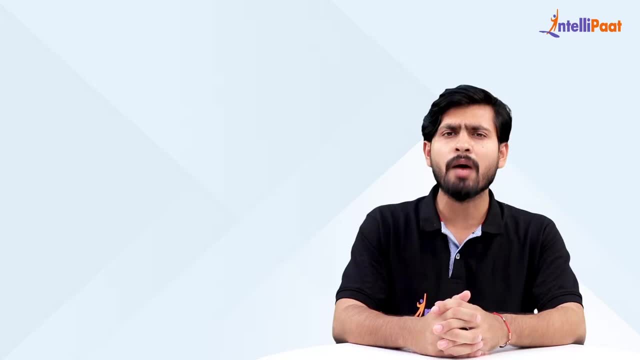 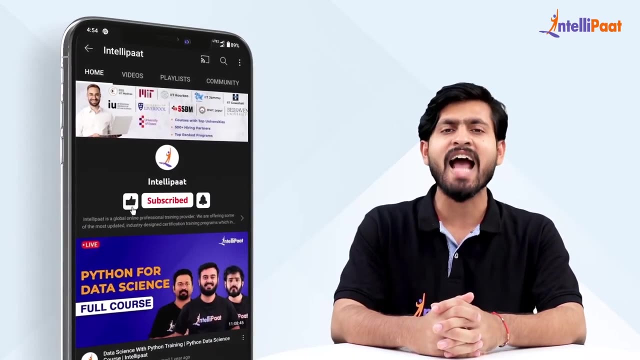 so amazing. no, Watch this video till the end to learn about what is data mining. But before we discuss our today's agenda, do not forget to hit the subscribe button and click the bell icon. First, we are going to discuss about what is data mining. Then 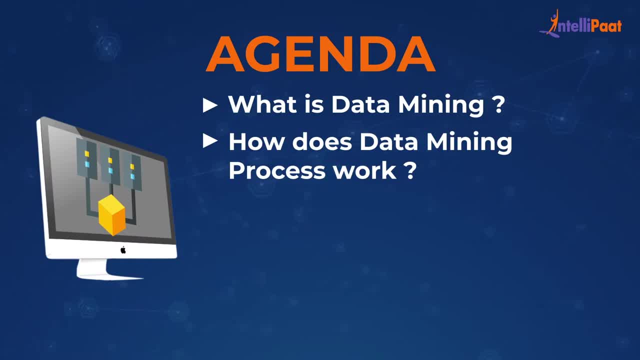 we are going to learn about how does data mining process work? Moving ahead, we are going to discuss about the data mining techniques. Then we are going to learn about the software tools required for data mining. Then we are going to learn about advantages of data mining. 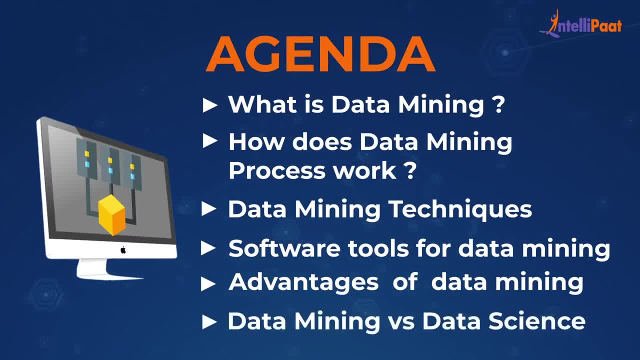 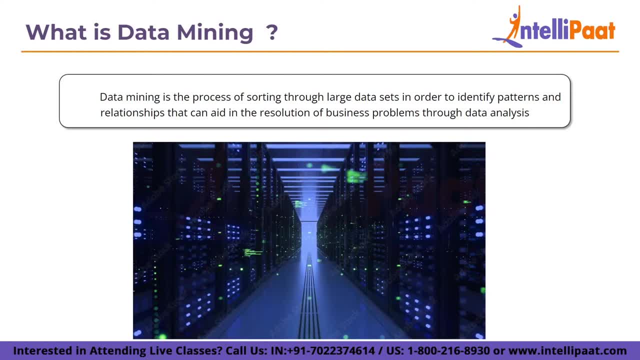 And at the end we are going to discuss about data mining versus data science. So let's start with: what is data mining? Data mining is a process of sorting through large data sets in order to identify patterns and relationships that can aid in the resolution of. 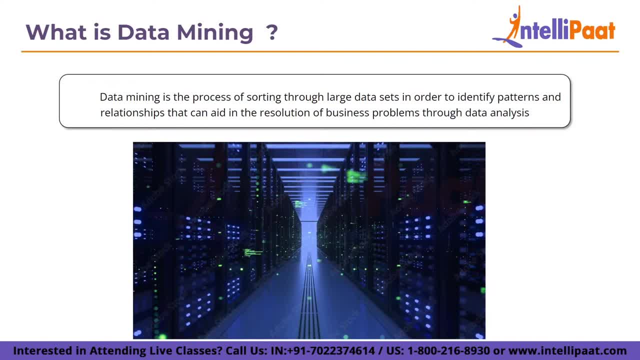 business problems through data analysis. Data mining techniques and tools enable businesses to forecast future results. Data mining is a process of sorting through large data sets in order to 대. ADD are sometimes used interchangeably, but they are more commonly regarded as distinct concepts. Now let's discuss. how does the data mining process work? 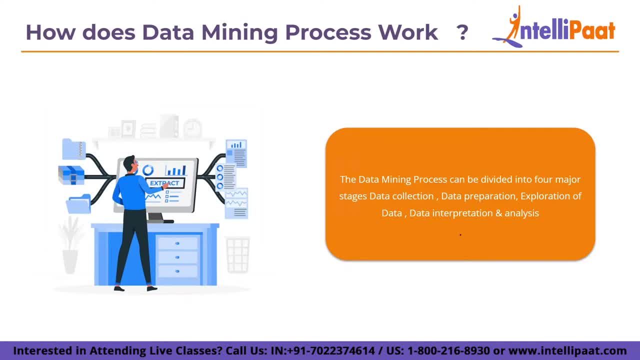 Data scientists and other skilled BI and analytics professionals are typically in charge of data mining. However, it can be done by data-savvy business analysts, executives and employees who act as citizen data scientists in an organization. Its main components are machine learning, statistical analysis as well as data management. 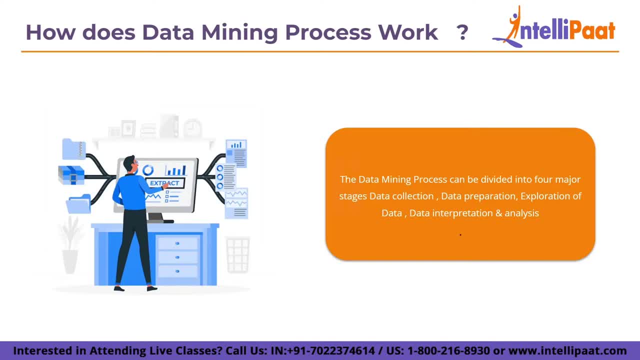 tasks performed to prepare data for analysis. The use of machine learning algorithms and artificial intelligence tools has automated more of the processes and made massive datasets such as customer databases, transaction records and log files from web servers, mobile apps and sensors. This is the first step in the process to make it easier to do the data-filtering process. 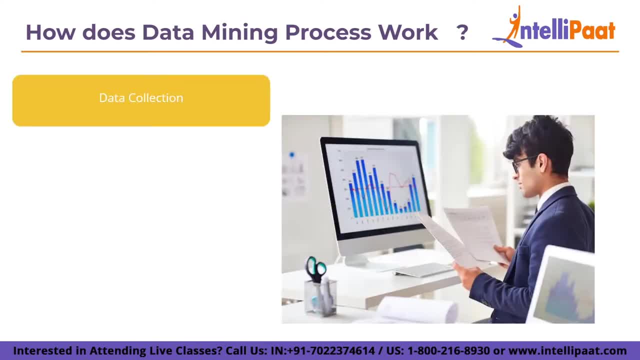 The data mining processes can be divided into 4 major stages: data collection, data preparation, exploration of data and data interpretation analysis. Let's discuss the first one, that is data collection. Data for an analytics application is identified and compiled. The data may be stored in various source systems: a data warehouse or a data lake. 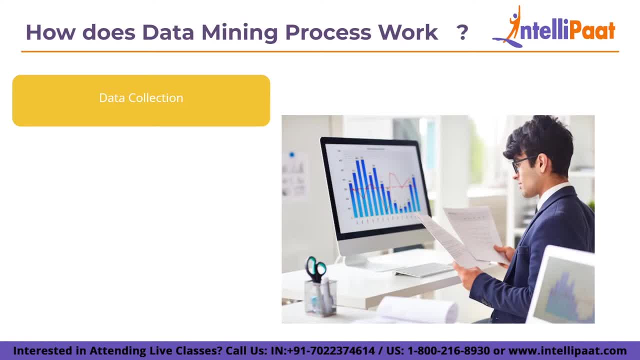 Data is stored in the database. The data is then stored in the database. The data is then stored in the database. data is then stored in the database. The data is then stored in the database lake, which is becoming an increasingly popular repository in big data environments containing. 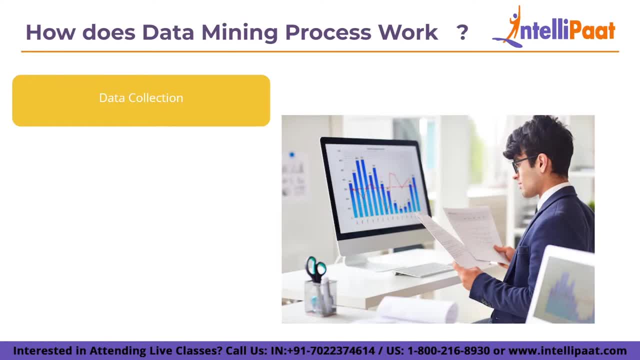 a mix of structured and unstructured data. External data sources may be also used as well. Regardless of where the data comes from, a data scientist will frequently move it to a data lake for the remaining steps in the process. Now let's discuss the second step, that is, data preparation. This stage includes a series 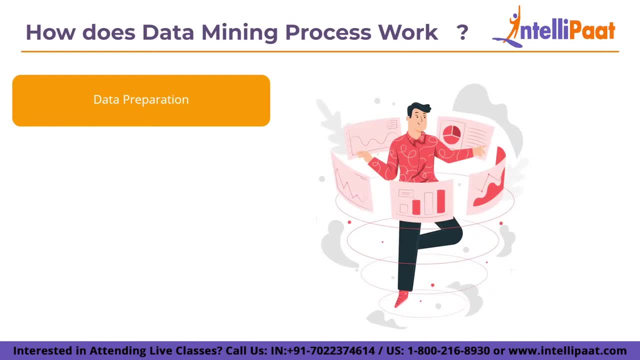 of steps that prepare the data for data mining. It begins with data exploration, profiling and pre-processing, and it is also followed by data cleansing work to correct sensors and other data quality issues, Unless a data scientist is looking to analyze unfiltered raw data for a specific application- data transformation. 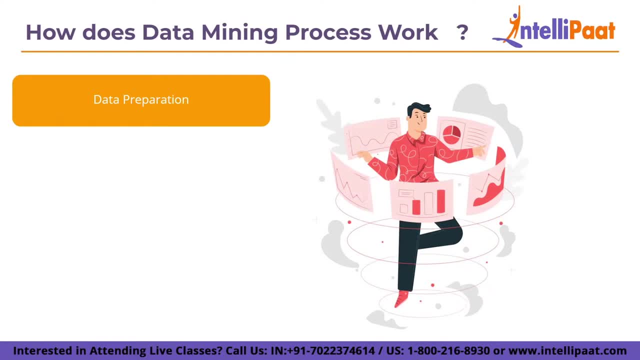 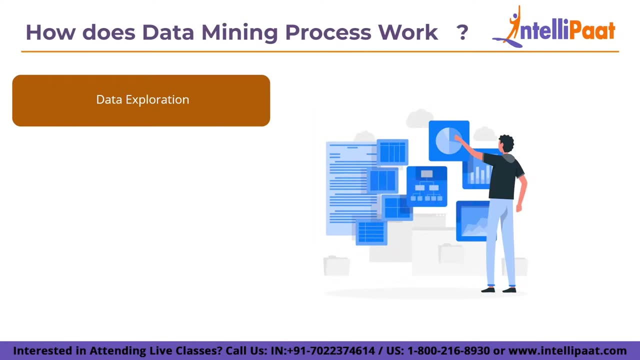 is also performed to make the datasets more consistent. Now next we have in the pipeline that is exploration of data. After preparing the data, a data scientist selects the appropriate data mining technique and then implements one or more algorithms to perform the mining In machine learning applications. the algorithms- 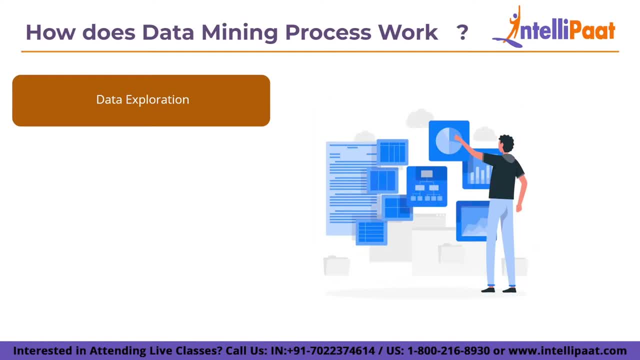 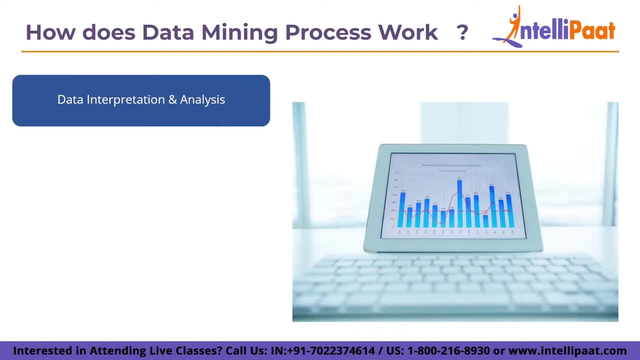 are typically trained on sample datasets to look for the desired information before being run against the entire sets of data. Next we have data interpretation and analysis. This is the final step. The results of data mining are used to develop analytical model that can aid in the decision making and other 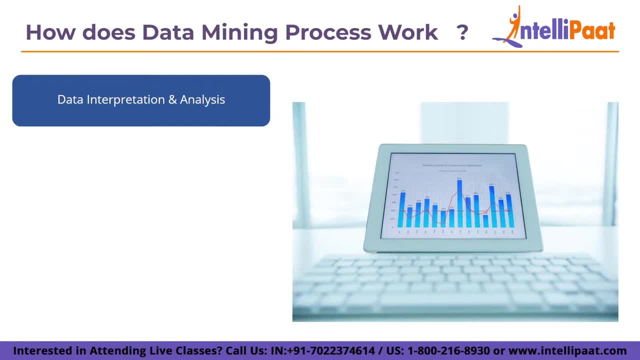 businesses action. The data scientist or another member of a data science team must also communicate the findings to business executives and the users, which is frequently accomplished through data visualization and data storytelling techniques. Now we have discussed all the four steps in the data mining process. Now let us discuss. 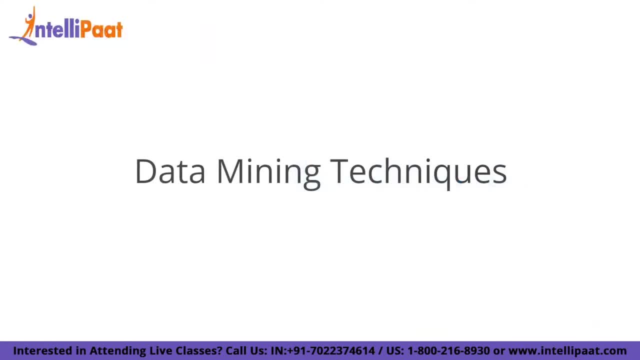 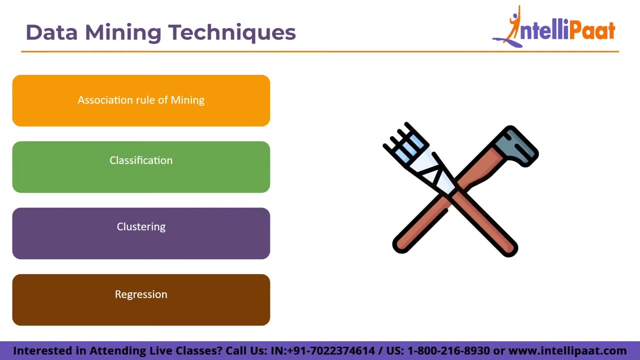 the data mining types of technique. To mine the data for various data science applications, various techniques can be used. A common data mining use case that is enabled by multiple techniques is pattern recognition or an anomaly detection, which aims to identify outlier values in the datasets. 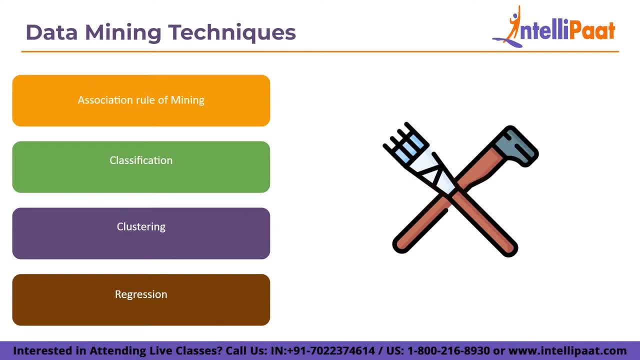 The following are few of the examples of the popular data mining techniques. The first one is association rule of mining. Association rules in data mining are if-then statements that identify relationships between data elements. To evaluate the relationships, support and confidence criteria are also used, And support measures helps us how frequently 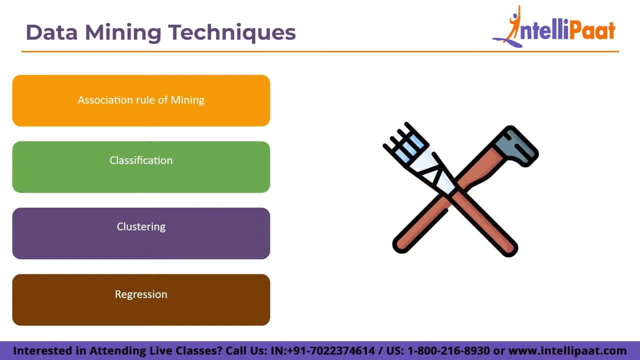 the related element appear in a dataset, While the confidence reflects the number of times and if-then statement is correct. Next technique we have in the pipeline is classification. This method categorizes the elements in the datasets using categories defined during the data mining process: Classification: 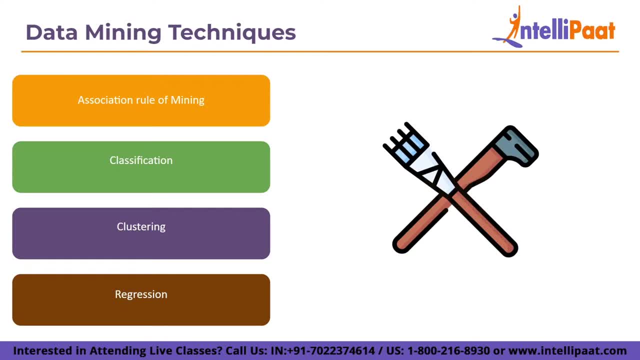 methods include decision trees, nape bias classifiers, k-nearest neighbor and logistic regression. Next technique which I am going to discuss is clustering. As a part of data mining applications, data elements with similar characteristics are grouped together into clusters. The few algorithms are k-means clustering, hierarchical clustering and Gaussian mixture models are. 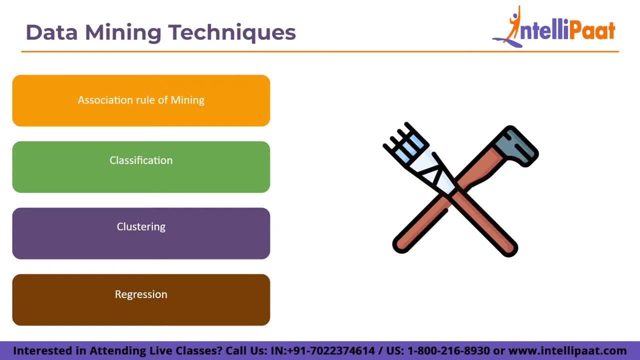 the few of examples. Next technique which we are going to discuss is regression. This is another method for discovering relationships in the datasets which is basically used to calculate the predicted data values based on set of variables- Example 1.. Examples include linear regression and multivariate regression. Regressions can also be performed. 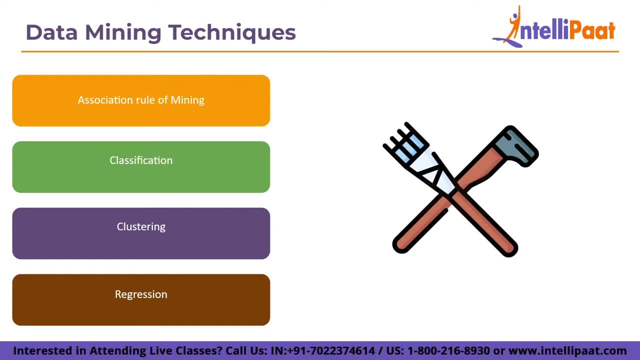 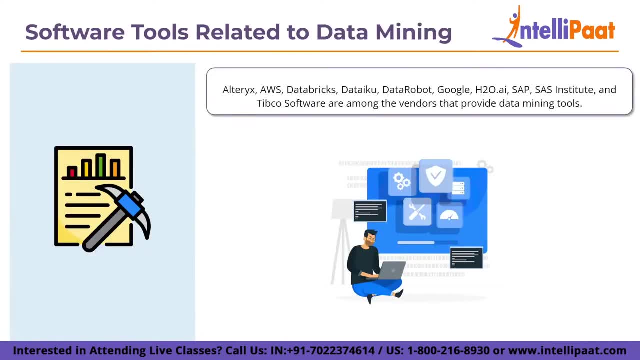 using decision trees and other classification methods. Now let us discuss the software tools for the data mining. Data mining tools are available from a wide range of vendors, usually as a part of larger software platforms that include data science and advanced analytics tools. Data mining- 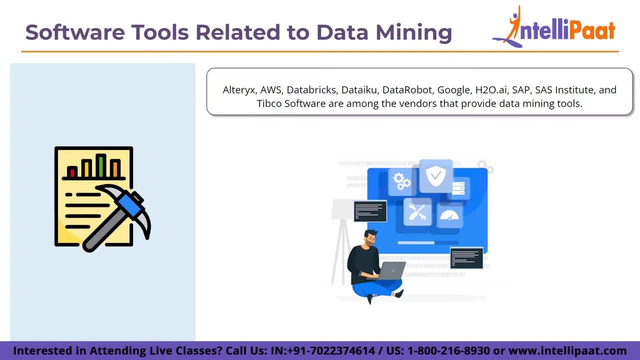 software's key features include data preparation capabilities, built-in algorithms, productive modeling support, a GUI-based development environment and tools for deploying models and scoring their performance. We have tools such as Alteryx, AWS Databricks, DataCube, DataRobot, Google H2Oai, IBM, KNMA and many more. 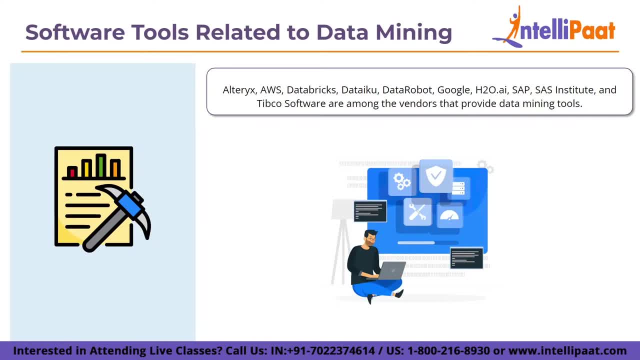 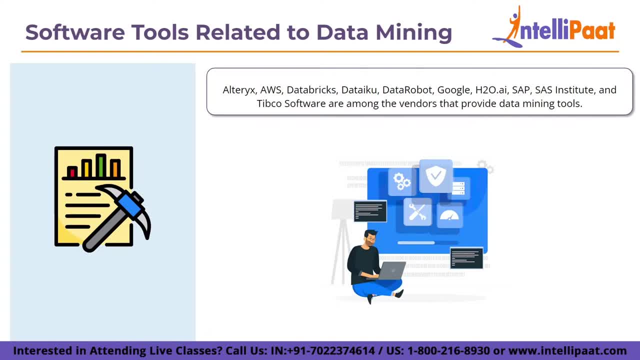 We have Datamilt, Elky, Orange, Rattle, Scikit-Learn and Veeca are a few of the tools in the pipeline. Some software vendors are also offering open-source options. KNMA, for example, combines an open-source 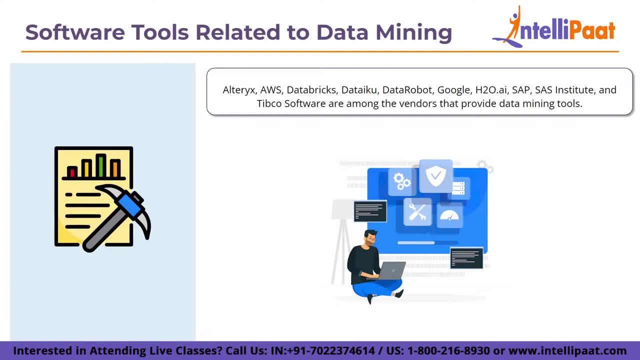 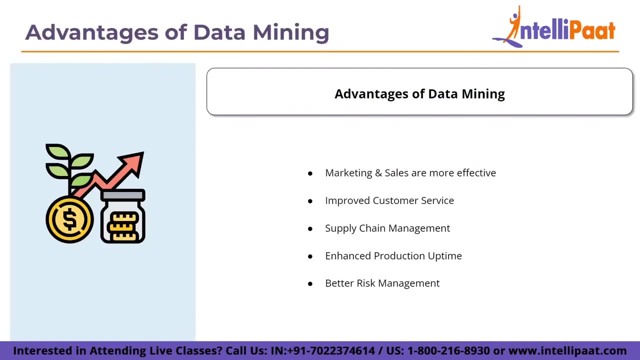 analytics platform with commercial software for managing data science applications, Whereas DataCаю and H2Oai provide free versions of their products. Now let us discuss the advantages of data mining In general: the increased ability to uncover hidden patterns, trends, correlations and 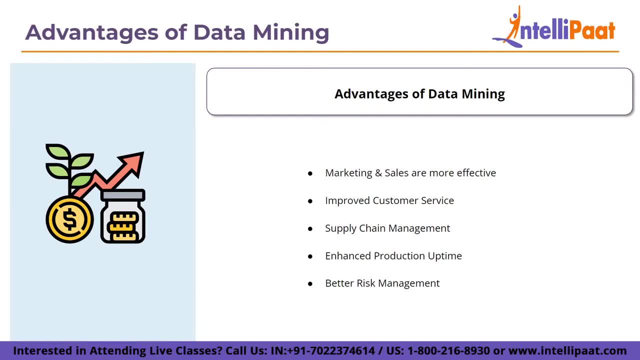 anomalies in the datasets results in business benefits. Through a combination of traditional data analysis and predictive analysis, this information can be used to improve business decision making and strategic planning. The following are some of the specific data mining advantages. The first one is marketing and sales become much more effective. 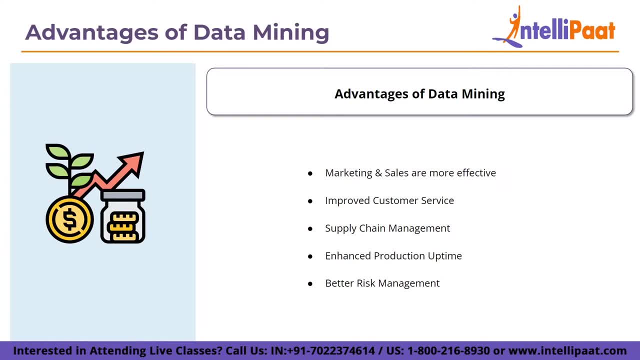 Data mining assists marketers in better understanding customer behavior and preferences, allowing them to create targeted marketing and advertising campaigns. Similarly, sales team can use the result of data mining to improve lead conversion rates and sell additional products and services to the existing customers. Now let us discuss the advantages of data mining. 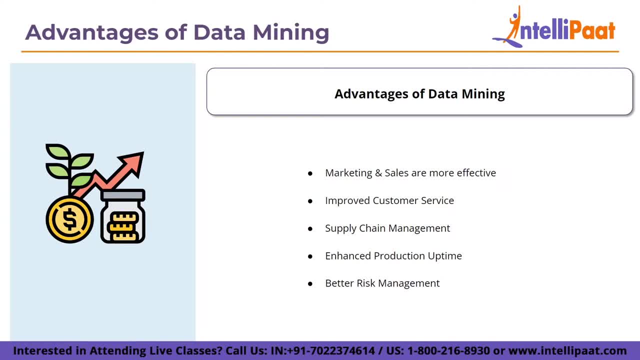 Next, we have improved customer service. Companies can use data mining to identify potential customer service issues more quickly and provide contact center agents with up-to-date information to use in-call and online chats with the customers. Next, we discuss of the advantage that is supply chain management. 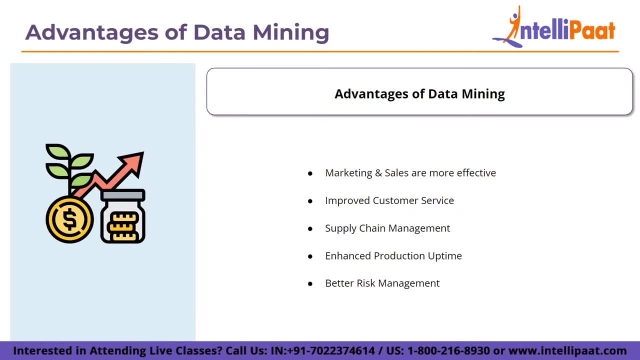 This has been also improved with the help of data mining techniques. Organizations can better spot market trends And forecast product demands, allowing them to better manage goods and supply inventories. Data mining information can also be used by supply chain managers to optimize warehousing. 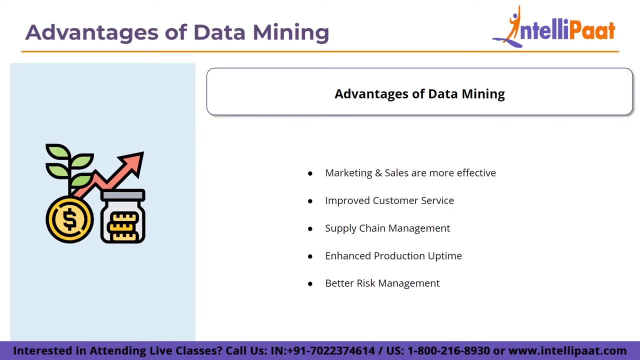 distribution and other logistics operations. Next advantage is enhanced production uptime. Mining operational data from sensors on manufacturing machines and other industrial equipment aids in productive maintenance of applications In identifying potential problems before they occur, thereby reducing unplanned downtime. Next advantage is better risk management. 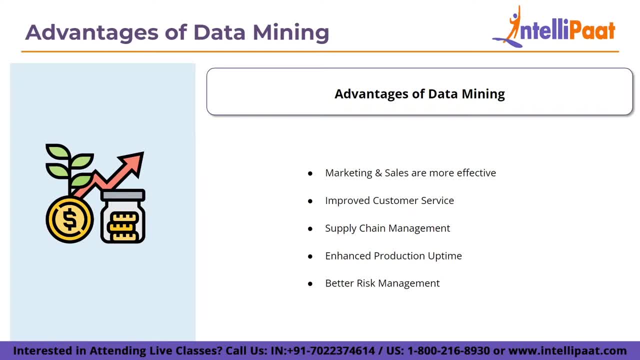 Risk managers and business executives can better assess and manage a company's financial, legal, cybersecurity and other risks. Reduced expenses also happen. Data mining contributes to cost savings by increasing operational efficiencies in business processes And decreasing redundancy and waste in the corporate spending. 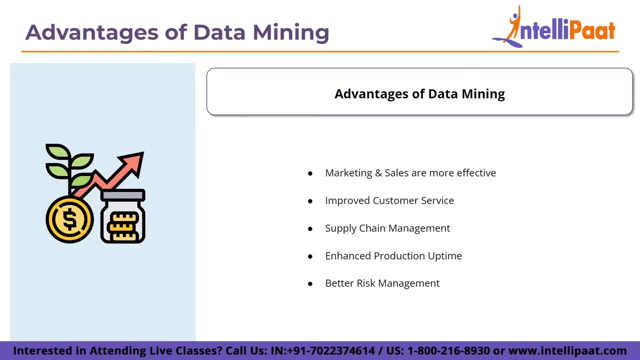 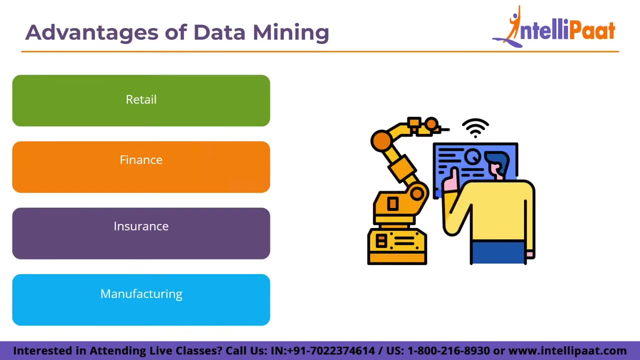 Finally, if I talk about data mining initiatives, it also leads to increased revenue and profits, As well as competitive advantages that distinguish companies from their competitors. Now let me give you some of the data mining industry examples. The first one is Retail Customers' data and internet clickstream records are mined by online networks. 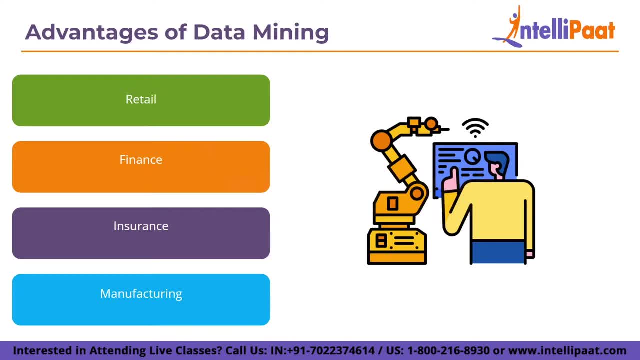 The first one is Retail Customers' data and internet clickstream records are mined by online networks. The second one is Retail Customers' data and internet clickstream records are mined by online networks. The third one is diesease-2021,, which is a number of marketplaces. 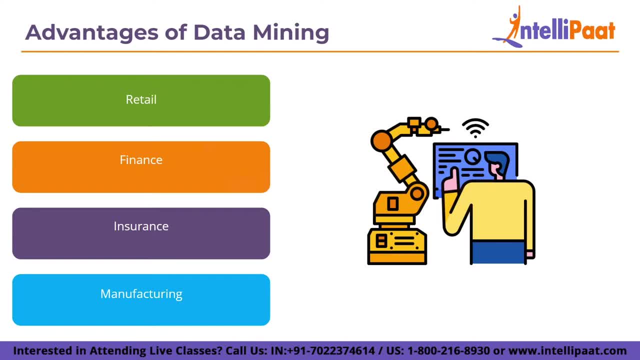 It's the first one of the greedy neighbourhood of perspective. It polished preferences from resellers to retailers to help them target marketing campaigns, nas and promotional offers to specific shoppers. Data mining and predictive modelling are also used to power recommendation engines that suggest potential purchases to website visitors, as well as inventory and supply chain management. 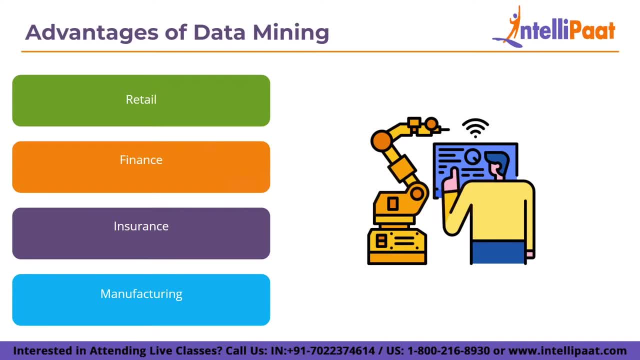 activities. If we look at another industrial example where we can find the benefits of using mining data is just services in finance: Financial use offers to the interface as well as other unexpected services. It's an interesting investment strategy where the platform also centers involved in今回's. 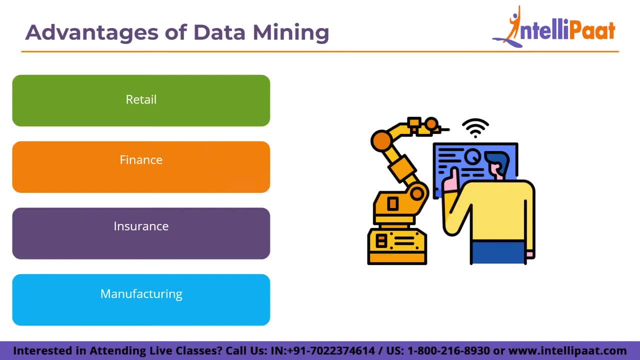 financial management. mining tools are used by banks and credit card companies to build financial risk models, detect fraudulent transaction and wait loan and credit applications. Data mining is also important in marketing and identifying potential upselling opportunities with the current customers. Next example: we can talk of using data mining in insurance companies. Data mining is used by 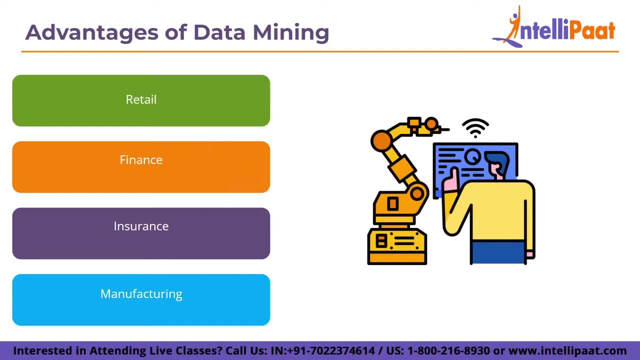 insurers to help them price insurance policies and decide whether to approve policy application, including risk modeling and management for prospective customers. Next example we can give of manufacturing sector: Manufacturers use data mining applications which help them to improve uptime and operational efficiency in manufacturing plants, supply chain performance and product safety. 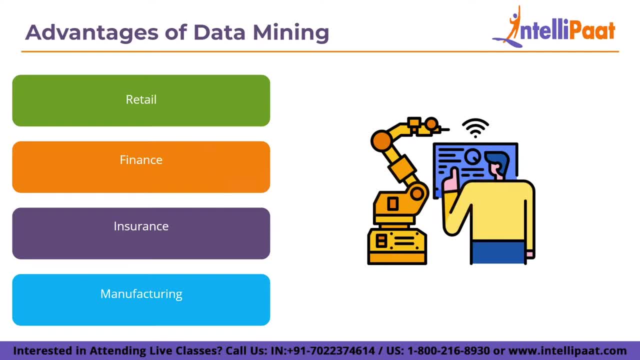 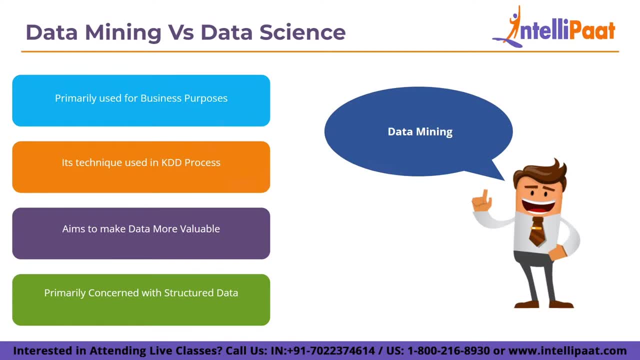 Now let us discuss what is the difference between data mining and data science. Data mining is a process that extracts useful information, patterns and trends from large databases that go beyond sample analysis and presents relevant and usable information that can be used to solve businesses problems. 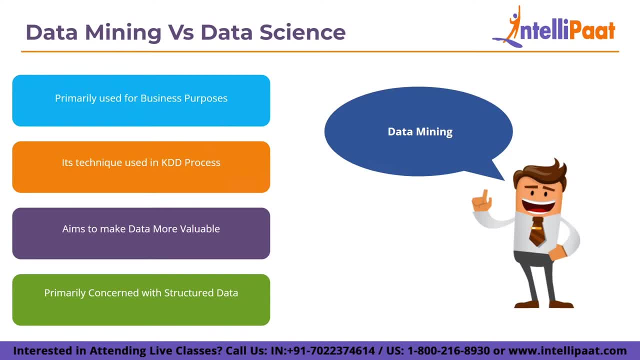 Whereas data science, on the other hand, is defined as a process of obtaining values, insights, from structured and unstructured data. how data science is harmful. If we talk about the differences and the different properties of data versus data mining and science, we can use certain parameters. 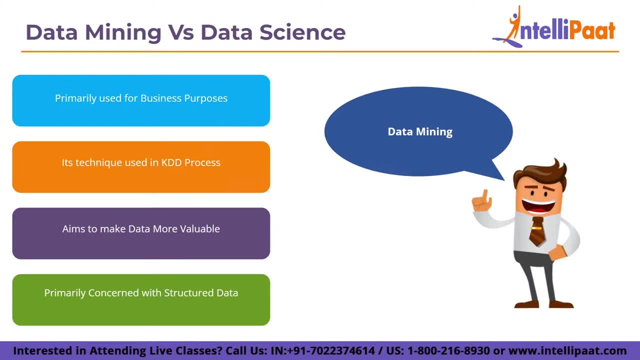 The first one is defining what is data mining. Data mining is the use of extraction of useful information, patterns and trends from our databases. It is primarily used for the purposes of businesses. Data mining aims to make datastronger valueable and usable.